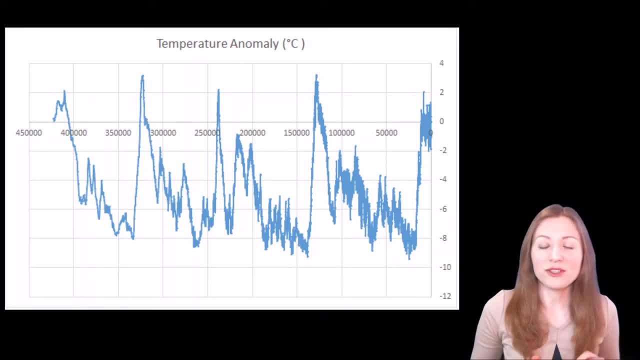 geological history. let's take a look at some of the most important glaciers in the world. In the section number two of your lab, you will build a graph similar to this one. In this graph you can see a difference in temperature from median values for about 450,000 years. 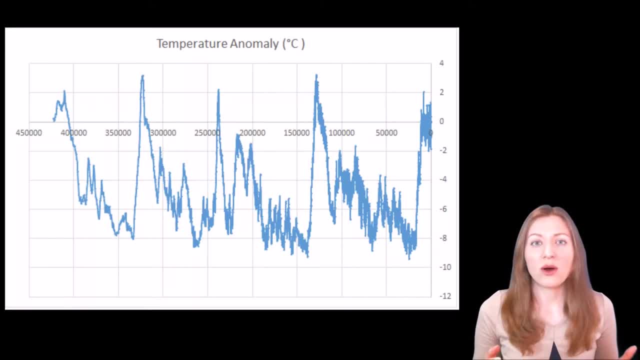 Zero in this graph means current time or average temperature. Please pay attention to this point. Zero in this graph doesn't mean zero Celsius or Fahrenheit, It's just the average temperature point. Temperatures kept below zero, from zero to minus 10,, indicate the glacial period or periods of. 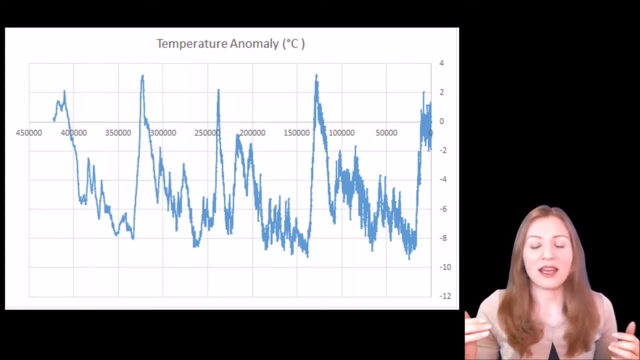 lower than average temperatures And the area above zero indicate interglacial periods or periods with higher than average temperatures. Some questions of your lab ask you to calculate an average difference in temperature or time. Considering that we're talking about geological time scale, you don't have to calculate the exact. 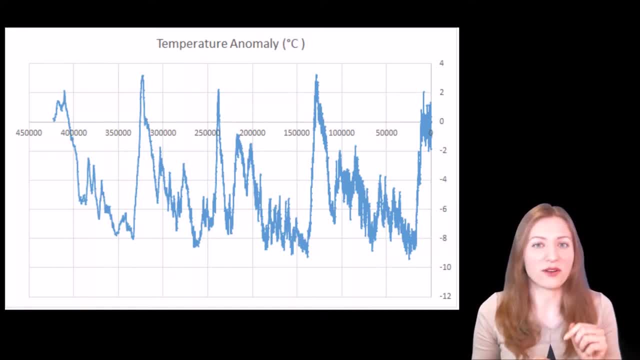 number of the average difference. Just take a look at the graph and notice that the average time difference between peaks of the glacial or interglacial periods is somewhere about 100,000 years. Scientists knew about colder and warmer periods in the Earth's history for a long time. However, nobody knew about cooler and warmer periods in the Earth's history. for a long time, However, nobody knew about colder and warmer periods in the Earth's history. for a long time, However, nobody knew about colder and warmer periods in the Earth's history. for a long time, However, nobody knew. 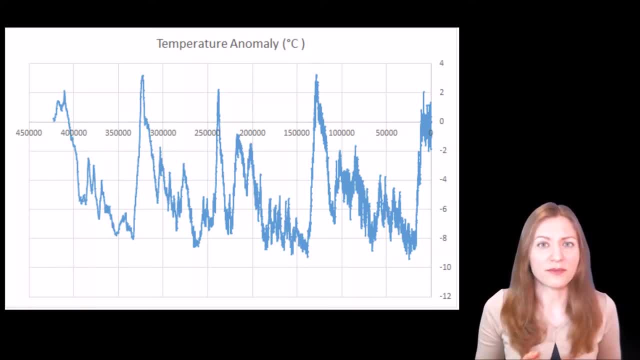 why such dramatic changes occur. until in the beginning of 20th century, Serbian astronomist Milutin Milankovic explained this mystery by his mathematical theory of climate. he showed that regular changes in Earth's orbit result in periods of lower temperatures on Earth, which correspond with the ice ages, the 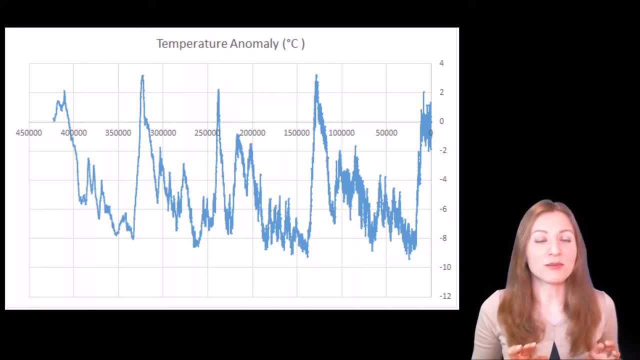 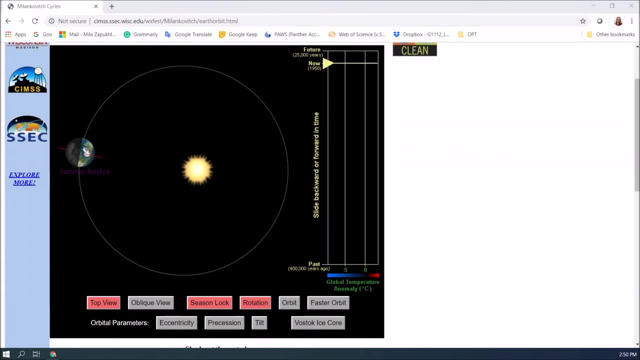 interactive visualization in the next slide will help you to understand his theory. this visualization represents a model of Milankovic cycle. first, you need to understand that this is only a model, so elements in it and distance between them are not shown to scale. what you need to explore in this lab are three.